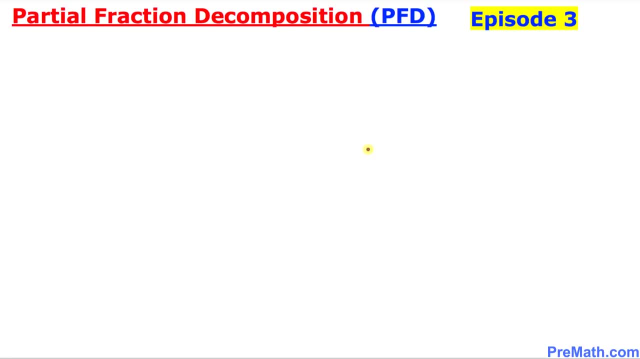 Welcome to Pre-Math. In this video tutorial, our topic is partial fraction decomposition, and this is our episode number three, And this time we will be discussing case number three. In this case, the denominator contains quadratic factors, And here are some of the examples that we're going to be dealing with. They belong to this case number three. Let's look at: in the very first example, this part is quadratic and this is irreducible. Once again, this part is quadratic. Quadratic means the highest power is two, and likewise this is quadratic as well. 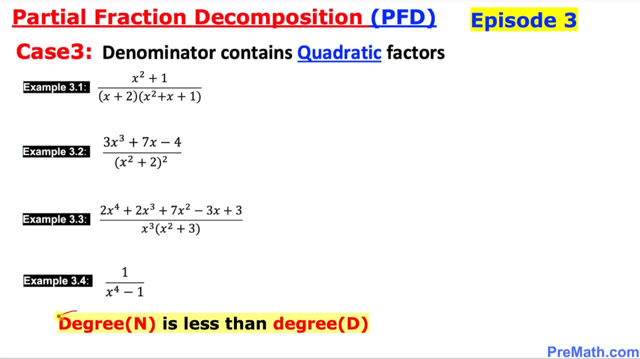 And one more thing: just keep in your mind that the degree in the numerator must be less than the degree in the denominator. And, as you can see, in all of our these examples, the degree in the numerator is indeed less than the degree in the denominator. 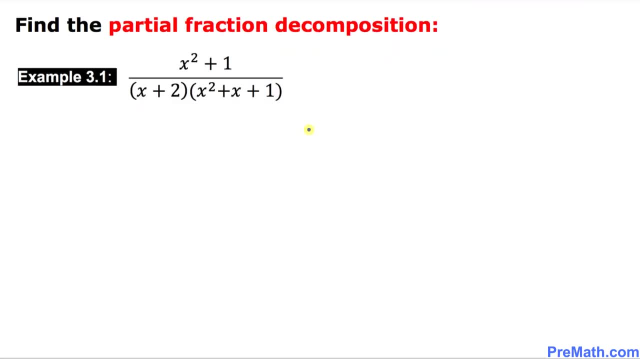 And here is our very first example, and we are going to find the partial fraction In the fraction decomposition of this rational expression. we again are going to focus on the denominator part. As you can see, in the denominator the first factor is obviously linear and the second one is quadratic. So we have two factors. That means we are going to get two fractions, The first one plus the next one. Okay, 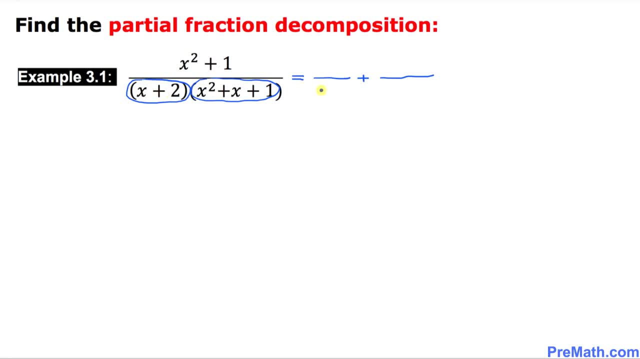 So now for the first one one, since this is a linear, so I am going to just put down x plus 2 over here. and the next one is quadratic, since its highest power is 2. we call it quadratic, by the way. and then the next step. 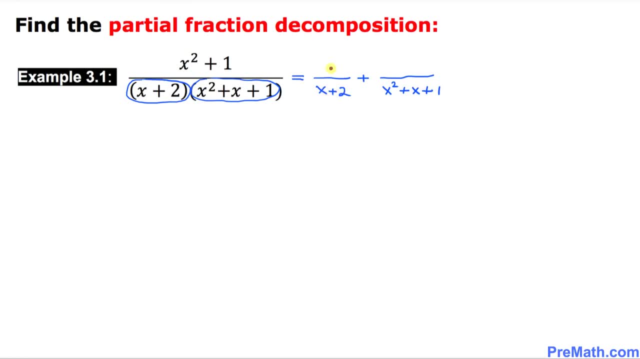 you know, whenever we are dealing with the linear, we always put a. I'm sure you learned it from your previous episodes. and as far as the quadratic factor is concerned, we always put B, X plus C. always remember that is going to be the case when we are dealing with the quadratic factor, and here 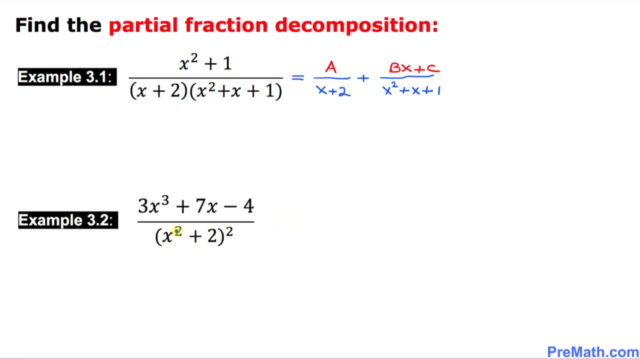 is an. our next example: we in the denominator have got this quadratic factor which is repeating twice. that means we are going to put two fractions. okay, that's the very first thing we are going to do. so I'm going to put down, as you know, when it's repeating twice, we're going to put down on D with: 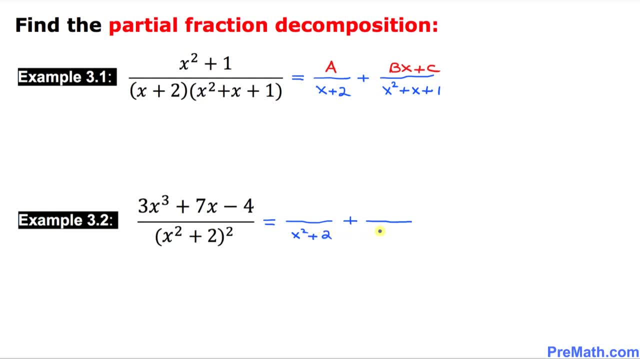 x square plus 2- power 1 first, and then the next time is going to be x- power 2 plus 2- power 2. all right, the next step is, since we are dealing with the quadratic factor factors, so this is going to be the first one- is going to be a: x plus b, always remember. 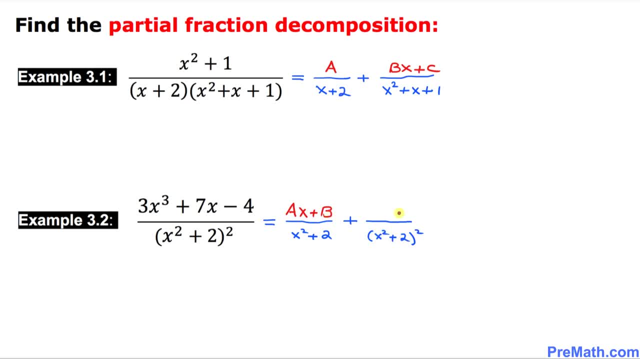 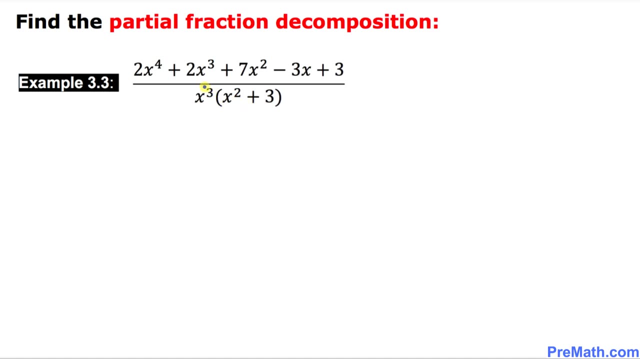 some constant time, x plus another constant, and likewise for this one is going to be c, x plus d. and here, in our next example, once again we are going to focus on the denominator and, as you can see, we have a one independent linear factor: x power three. that means it is repeating itself three times. and the next one: 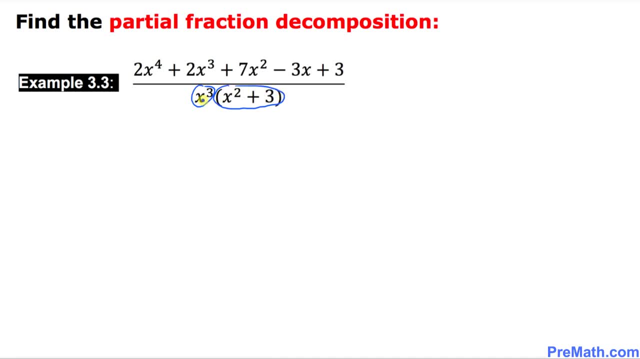 is quadratic factor. so that means all together we're going to have four fractions, so i'm going to put down first one plus always put a plus sign in between each fraction. three fractions plus another one. all right, the very first thing is, let's focus on this linear factor: x power three. 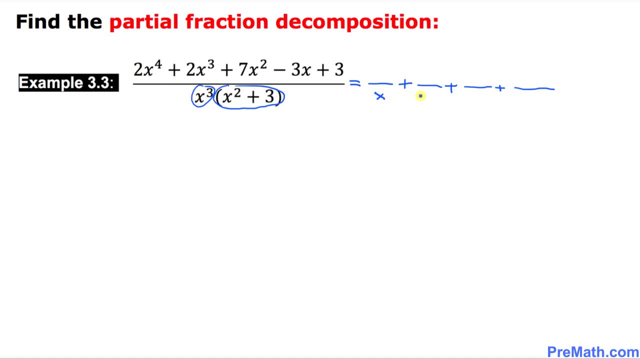 as you know, that the first is going to be x power one, then it's going to be x power two in the denominator, and then x power three when they are linear and when they are repeating themselves, and the second one is our quadratic factor. so i am going to put down x power two. 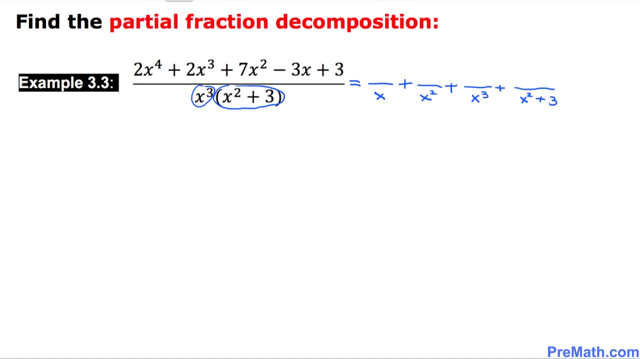 two, two plus 3.. Now let's take care of the numerator. So, since this is linear, I'm going to put simply an a constant, some constant a for this one. second fraction is going to be a b, third one is going to be a c, and for the fourth fraction, since this is a quadratic, so we have to be very careful. 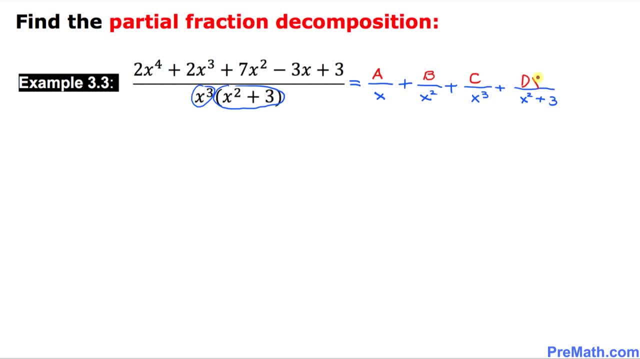 so this is going to become d x plus e. all right, and here is an, our final example. we are going to take care of this one. let's focus on the denominator part over here, which is x power 4 minus 1, and I have just copied down this x power 4 minus 1 right here. let me just show you. 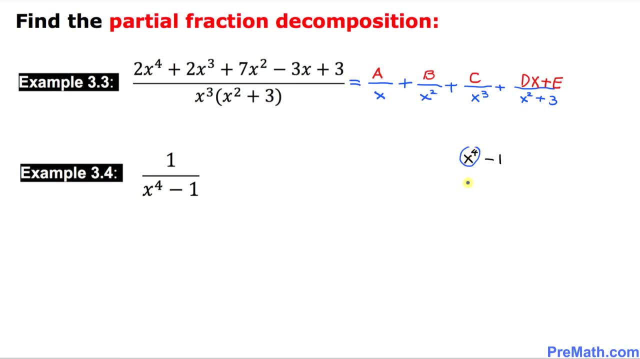 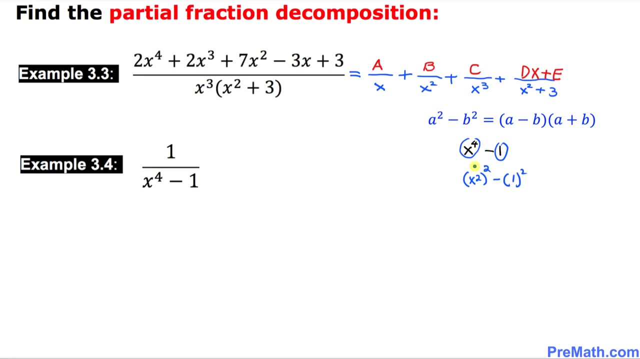 let's take a look at this one and let's see how it works. So this is going to be d x plus e. focus on this- x power 4. I can write x power 4 as x power 2, and then power 2 and 1 could be written as minus 1 square and now, as you can see, this represents: 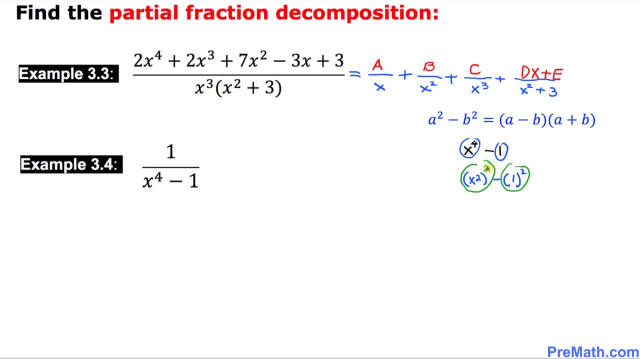 the difference of two squares. so we are going to be using this well-known fact. the difference are two square a square minus b square equal to A minus B times A plus B. that means I can write this one as X square minus 1 times X square plus. 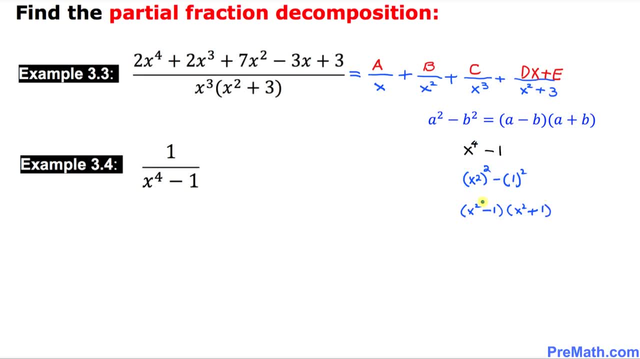 1. and now we are going to focus on the first parentheses. this part only X square minus x squared equal to B times A times a plus B. that means I can write minus 1, which could be written as x square minus 1 square. Once again, this represents a difference. 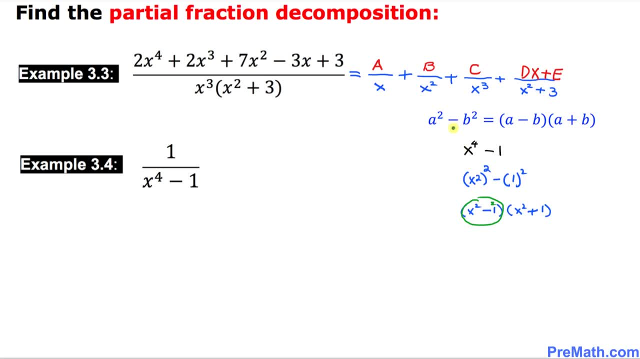 of two squares. We are going to be using the same fact: a square minus b, square equal to a minus b times a plus b. Let's go ahead and take care of that one, for this part only, So that's going to become simply x minus 1 times x plus 1, and we have already this thing here. I'm going to just bring. 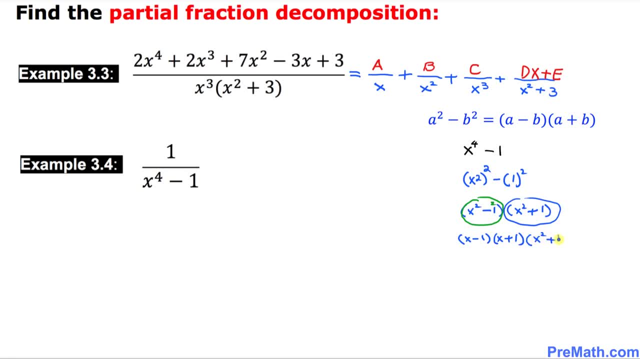 it down: x square plus 1.. So that means: so this is a complete factorization factors of this: x power 4 minus 1.. So that's it. This rational expression could be written as 1 over x power 4 minus 1.. The complete factors are: 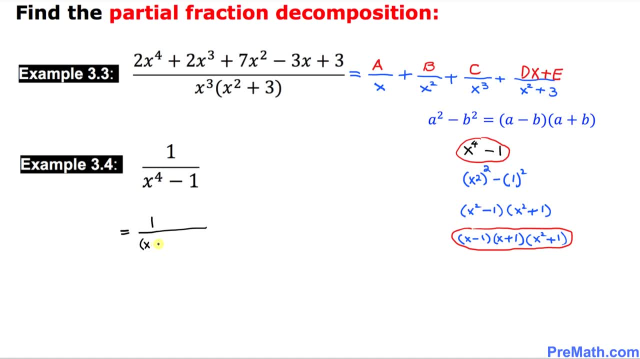 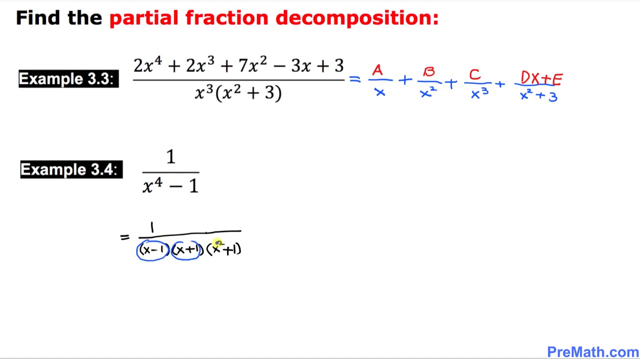 x minus 1 times x plus 1 times x, square plus 1.. So far so good. And now we can see in the denominator we got two linear factors and one quadratic. So we're going to have three fractions, one plus another, one plus another one. So first I am going to put down x minus 1 in the 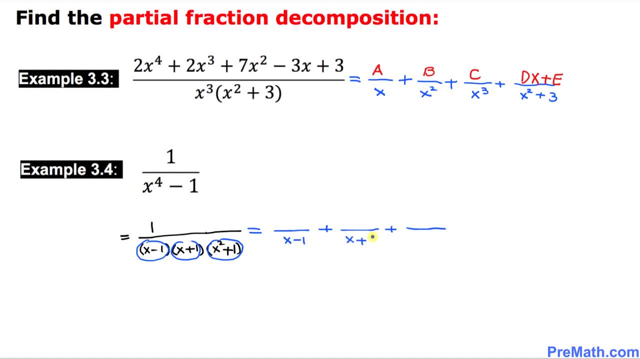 denominator, then x plus 1, and then x square plus 1.. And the next thing we are going to do is on the numerator, on the top part, for this first fraction is going to be a constant and then then it's going to be. the second one is: 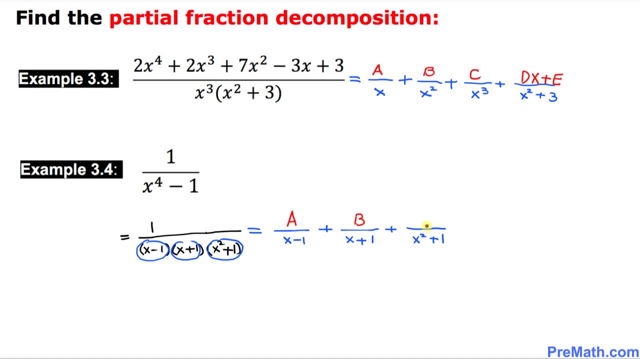 going to be b, and for the third fraction, since this is a quadratic, I'm going to put down c, x plus d. And now the next thing is how to find the value of these constants: a, b, c and d. I will show you in our next episode. and finally, here is our case number four. 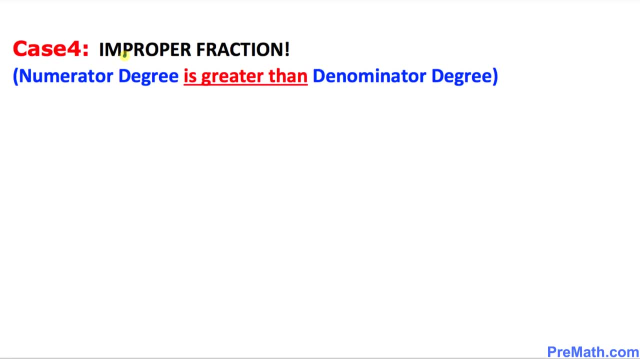 in this case we call is improper fraction. in other words, the degree in the numerator is always greater than the degree in the denominator. and here is the example: as you can see, in the numerator, our highest power, our highest degree is three, and in the denominator, the highest degree is: